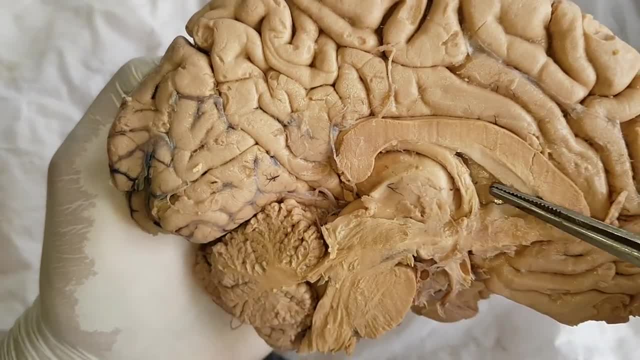 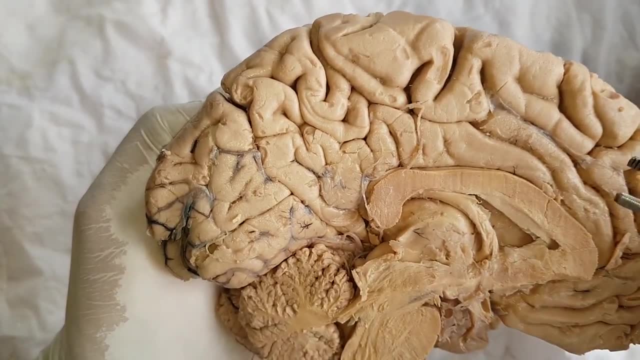 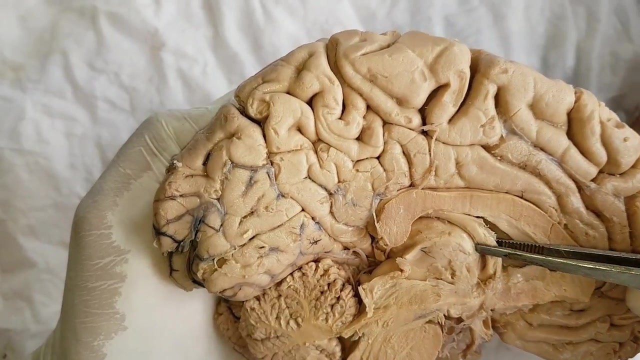 Then, just beneath this corpus callosum, you can see one cavity, and this cavity is the cavity of lateral ventricle. Then here you can see one more structure. this one is the body of fornix, and this body of fornix is the continuation of cross of fornix on. 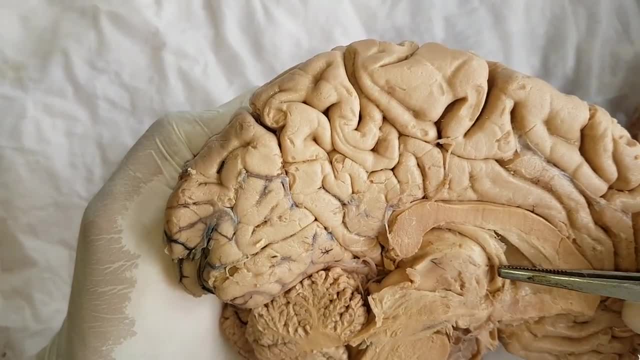 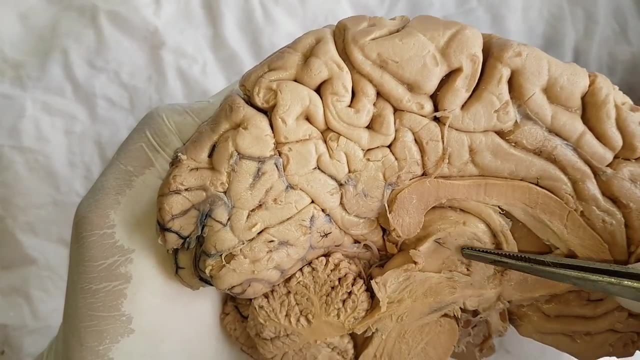 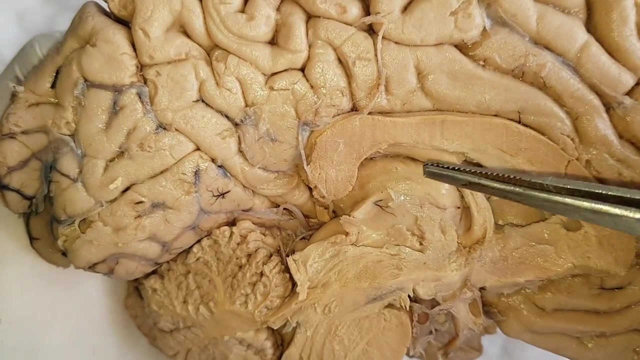 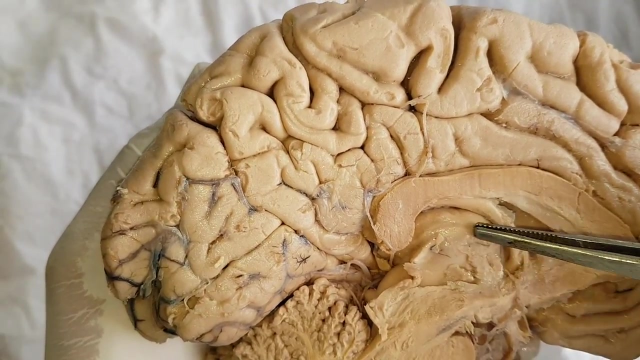 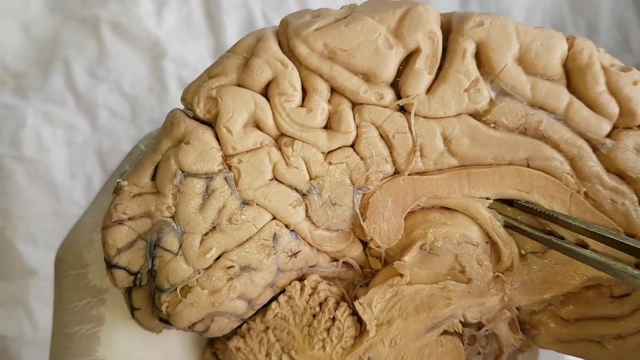 each side and this body of fornix anteriorly diverges into the columns. Now, here you can see one elevation, this one, and this elevation is the thalamus. You can see clearly this one, and this is the cavity of third ventricle, this one. So this cavity of third ventricle communicates with this cavity of lateral. 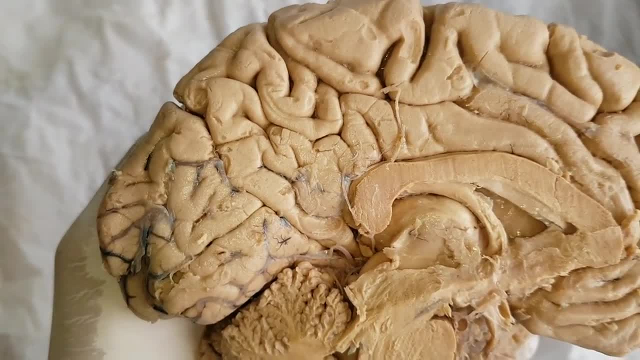 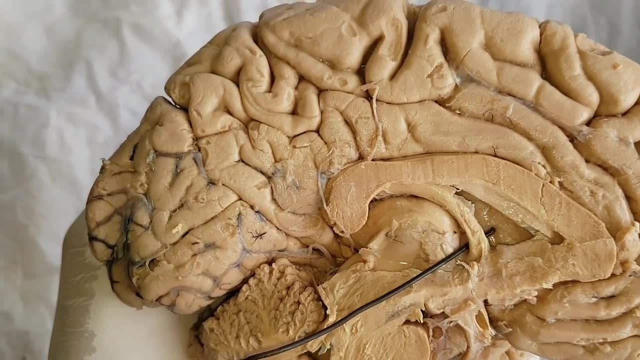 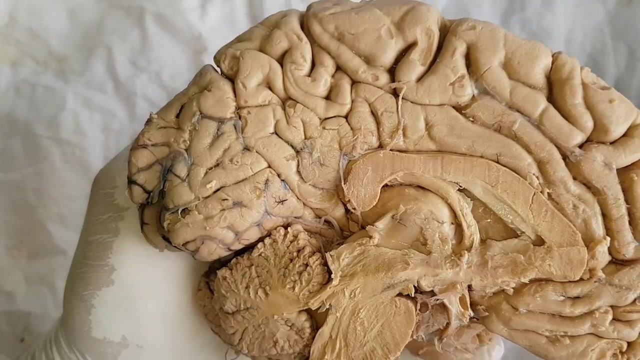 ventricle through a foramen, and this foramen is known as the interventricular foramen or also known as the foramen of Monroe. Here you can see this is the foramen of Monroe or interventricular foramen. Also you can see the brain stem. this one. 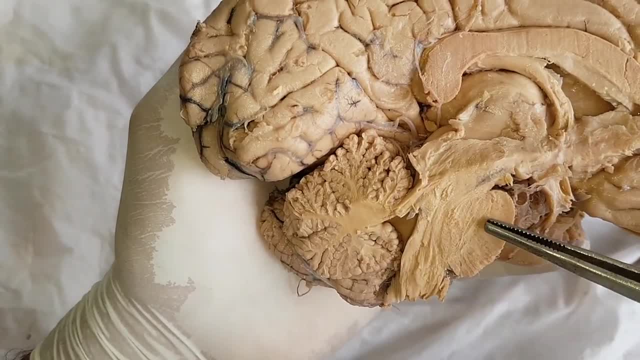 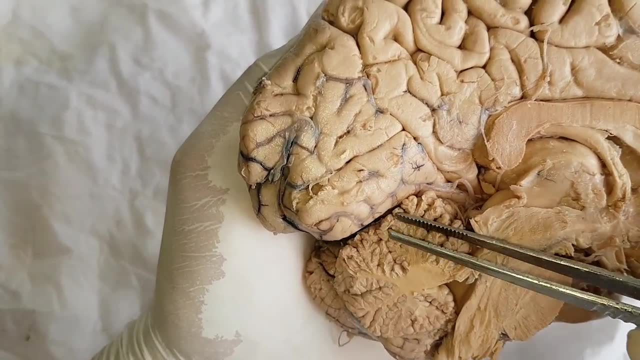 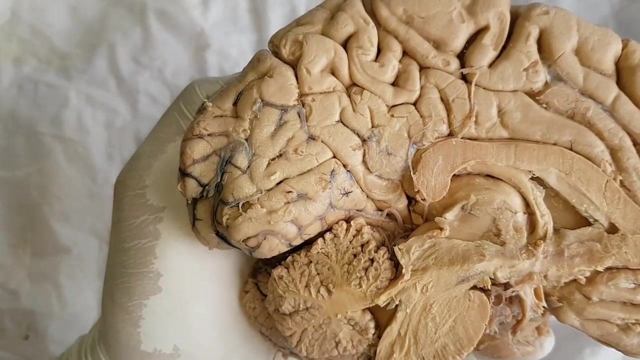 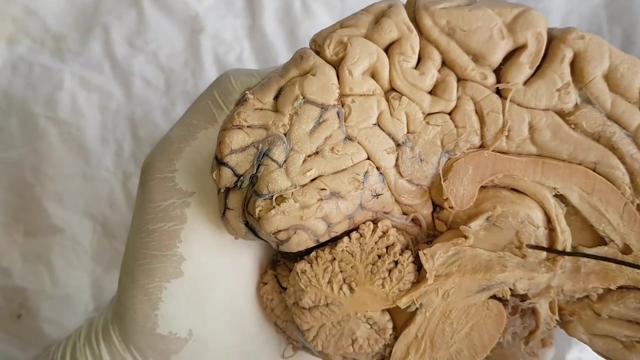 this is the midbrain, this is the pons and this one is the medulla. but this pons and the medulla are separated from this cerebellum by this cavity. this one, this, is the cavity of fourth ventricle and this cavity of fourth ventricle, this, communicates with this cavity of third ventricle. 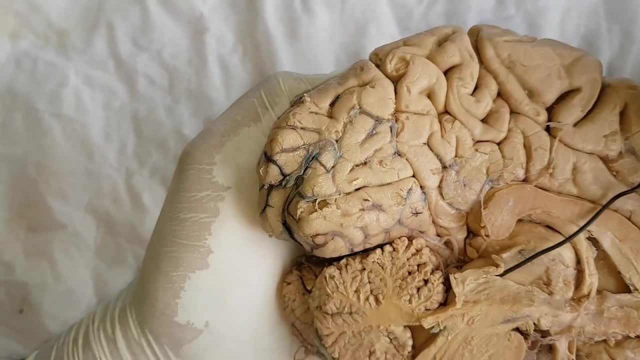 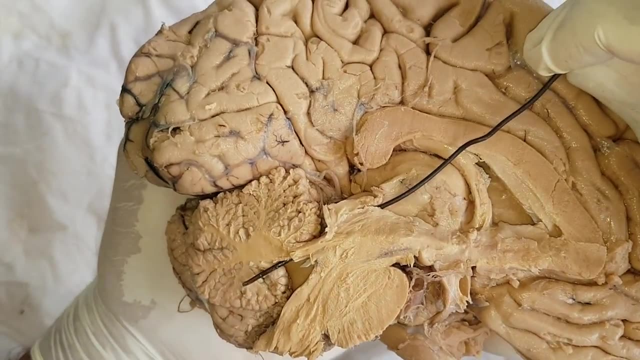 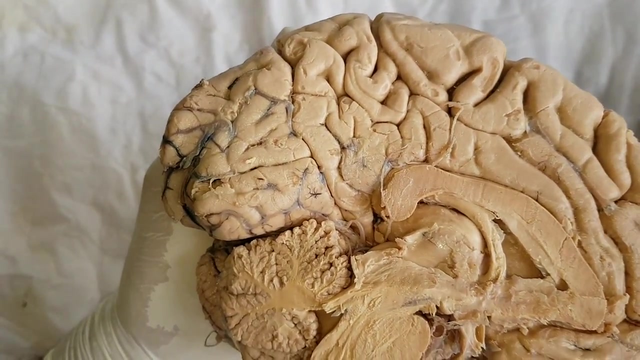 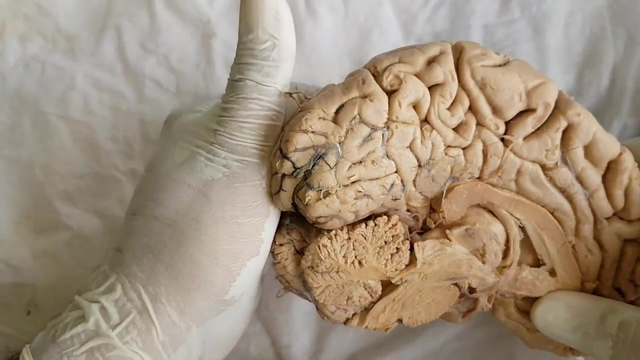 through a aqueduct of sylveus. so here you can see this is the aqueduct of sylveus. you can see clearly this is the aqueduct of sylveus. so this is all about the mid sagittal section. now we will see the coronal section now in this section, apart from this cavity of lateral 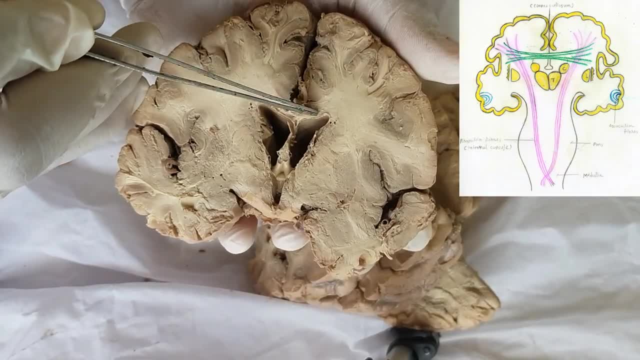 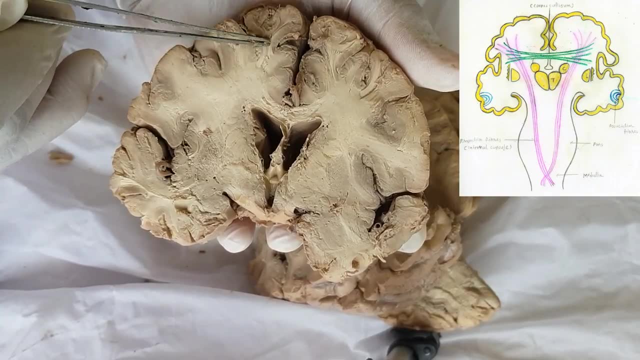 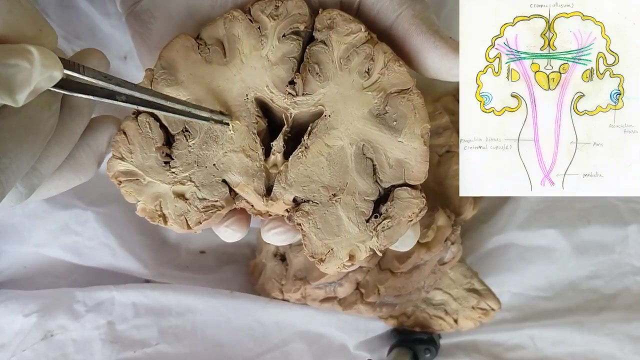 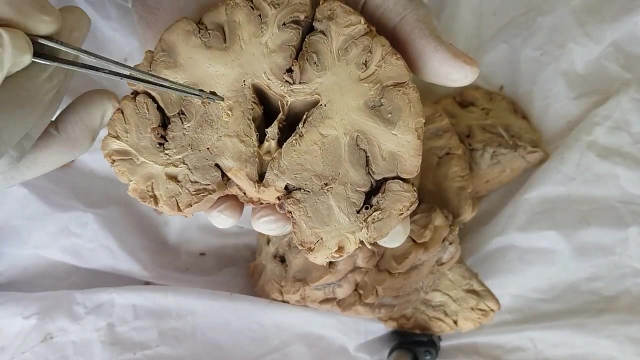 ventricle. you can also see these white fibers of corpus callosum which are the example of commissural fibers. then here you can see the white fibers of the corona radiata and these white fibers on each side, internal capsule, which are the examples of projection fibers. and here you can. 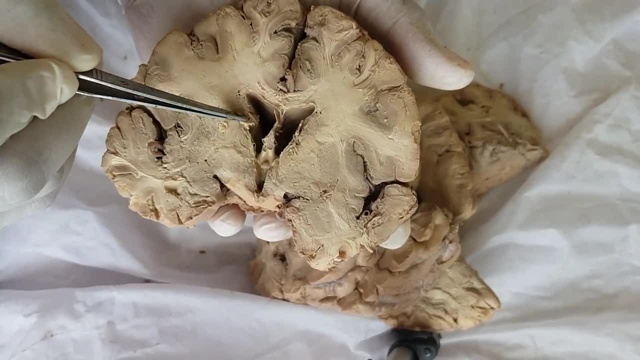 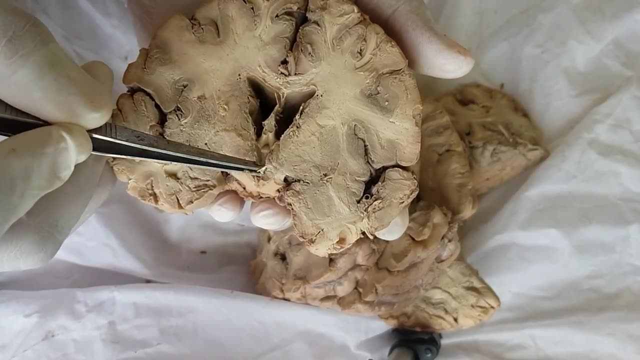 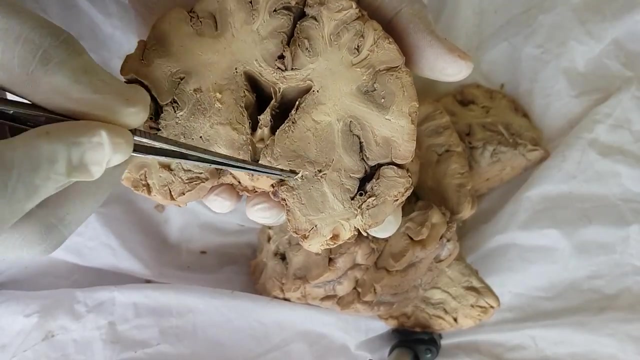 see the gray matter on each side is the caudate nucleus and here you can see, on each side of cavity of third ventricle, gray matter of thalamus, and here you can see gray matter on each side is the lentiform nucleus. now suppose i am taking a. 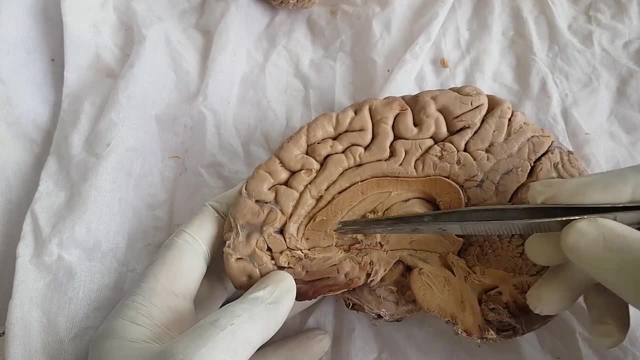 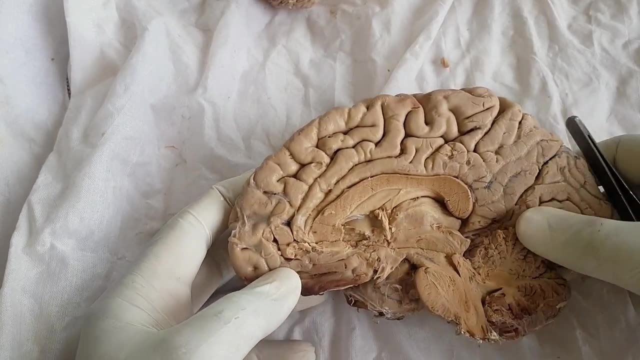 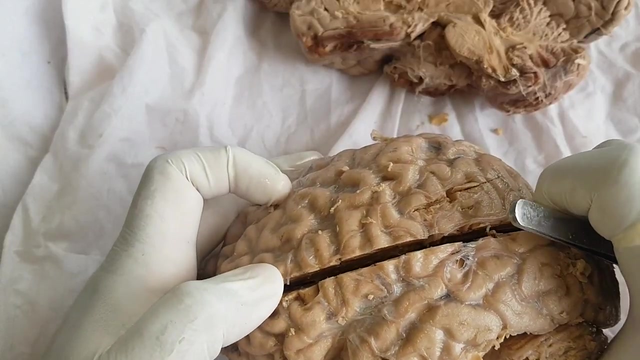 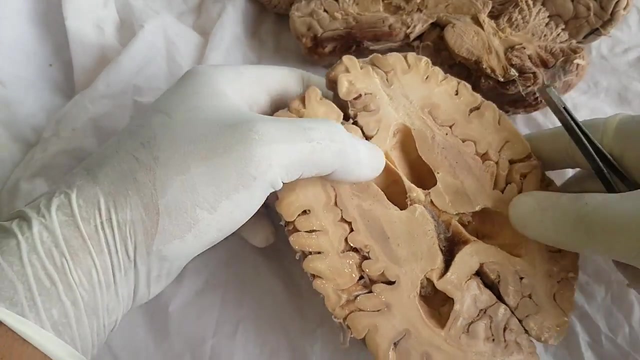 section at the level of this genu and the splenium of corpus callosum, like this transverse section, then how it is seen. so it is seen like. so here i am taking a transverse section, this one at the level of genu and the splenium of corpus callosum, so here you can see. 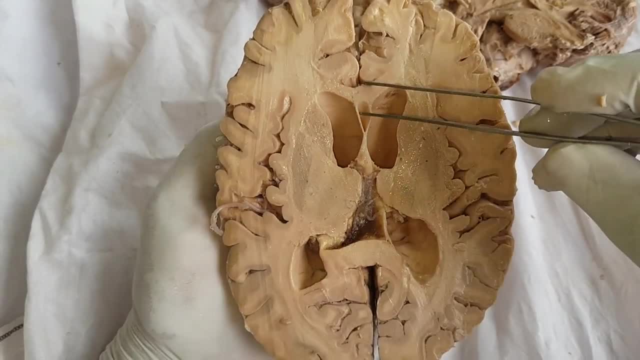 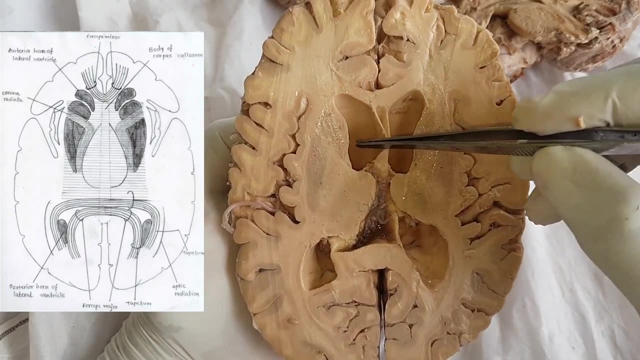 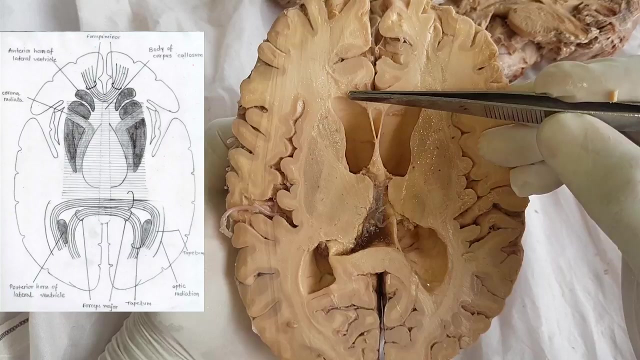 the video structures. so this is the genu of corpus callosum, this is the splenium of corpus callosum, here is the cavity of lateral ventricle and this is the growth of lateral ventricle on both side. so you can see the fibers passing through this genu of corpus callosum and these fibers are known. 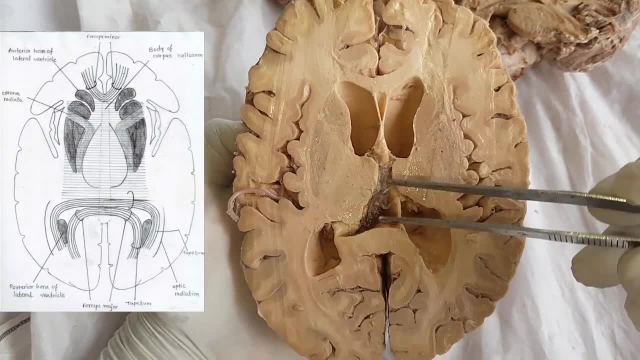 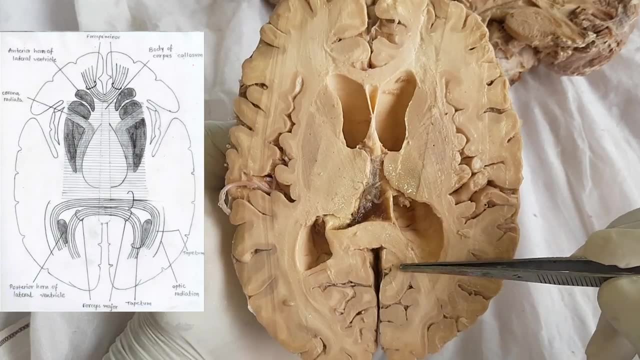 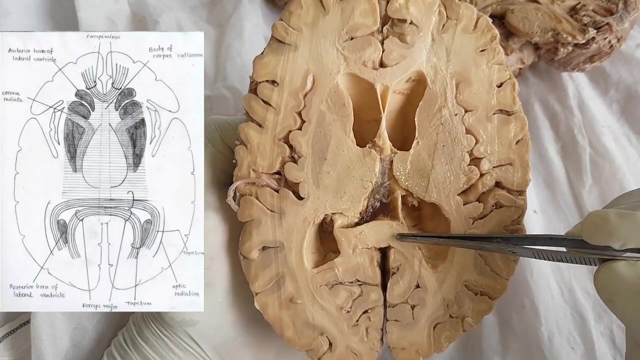 as the forceps minor connecting the frontal lobe of both side and fibers passing through this splenium of corpus callosum, and these fibers are known as the forceps major connecting the occipital lobes of both sides and these fibers of forceps minor. 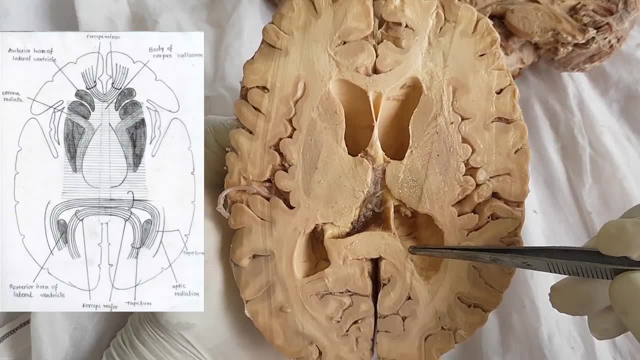 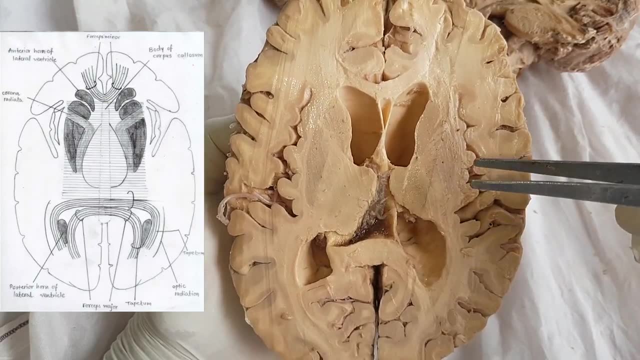 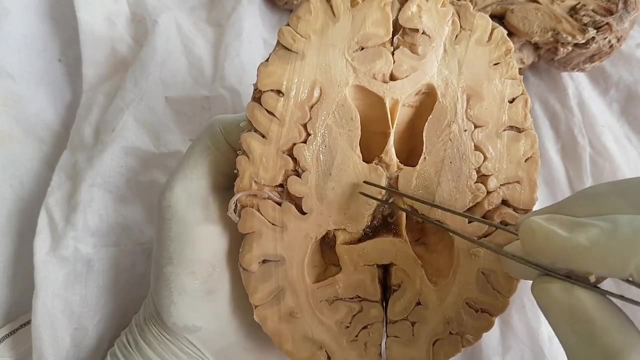 measure produce the elevation in the posterior horn of lateral ventricle. This is the posterior horn, known as the bulb of posterior horn. on both side Now here is the cavity of third ventricle. So on each side of this cavity of third ventricle you can see the thalamus. 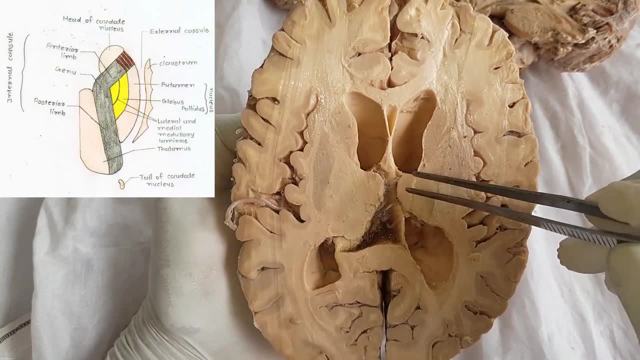 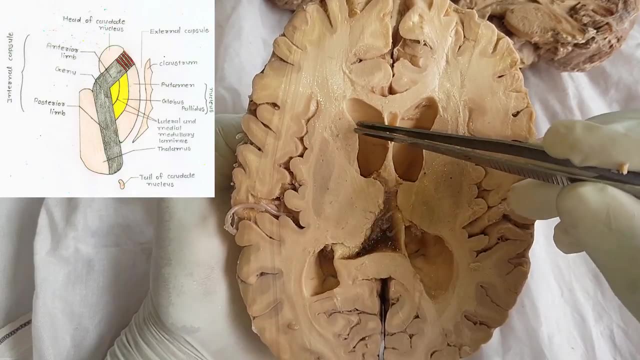 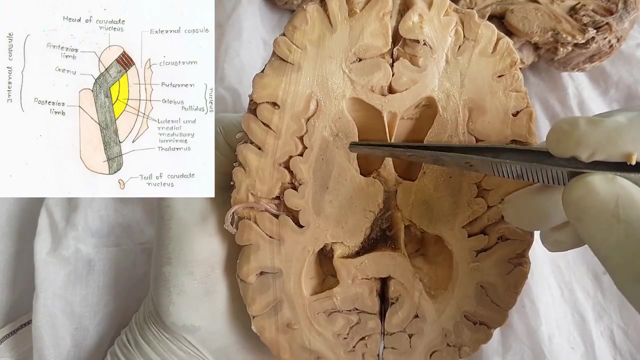 masses of gray matter on both side. Then here you can see: this is the caudate nucleus on both side, This one, this is the masses of gray matter. again Now, this caudate nucleus and the thalamus on both side, separated from the another: masses of. 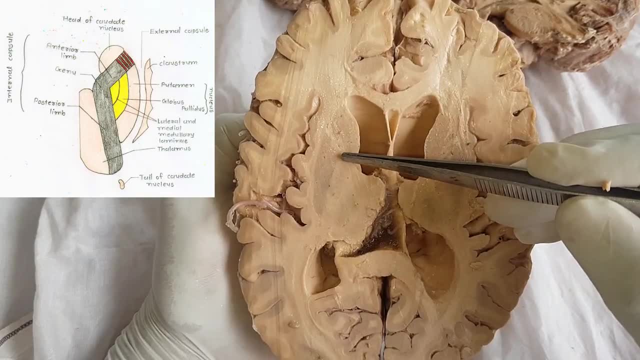 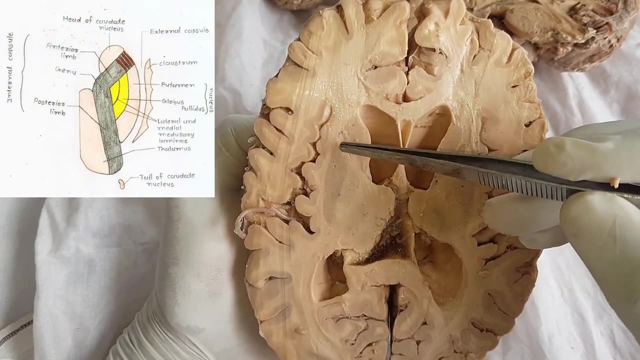 gray matter by this white fibers. You can see V-shaped white fibers And this is the internal capsule, this white fiber. Here is the anterior limb of internal capsule. Here is the anterior limb of the anterior limb of the anterior limb of the anterior limb. 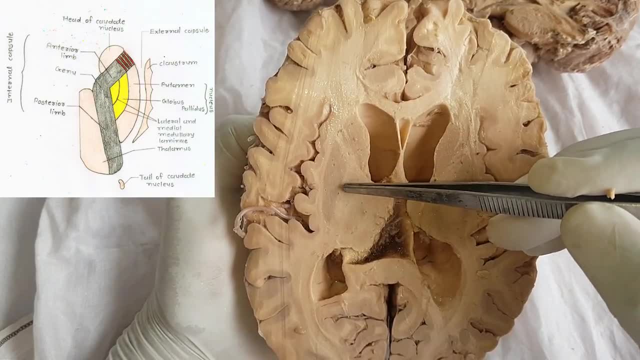 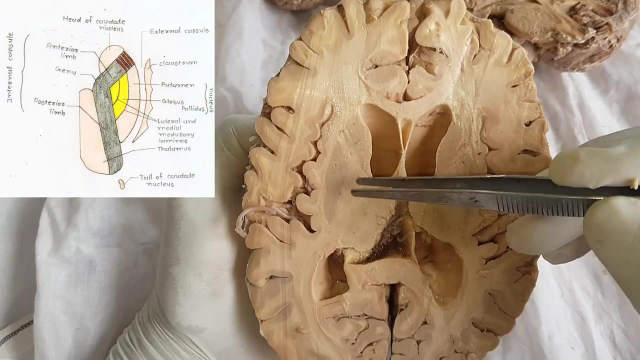 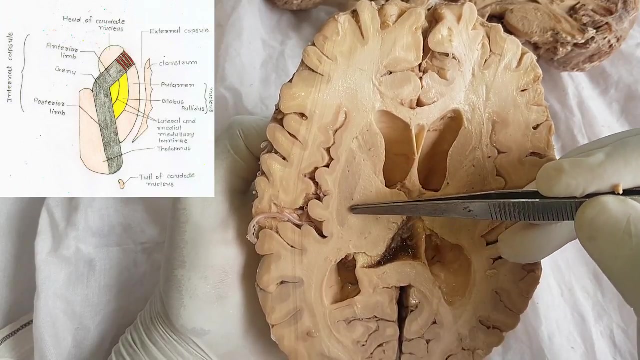 Here is the genoa of internal capsule and this is the posterior limb of the internal capsule which separate the caudate nucleus and thalamus from the another mass of gray matter. here you can see, and this is the lentiform nucleus, and this lentiform nucleus, again divided, 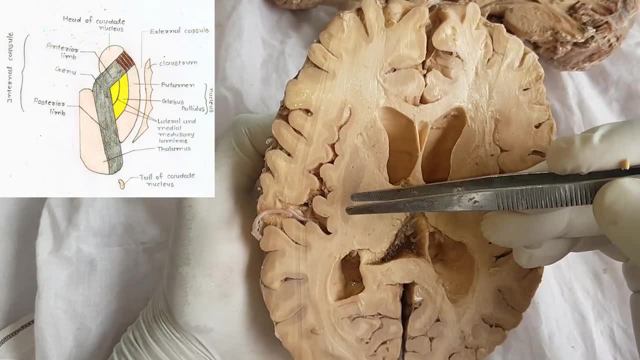 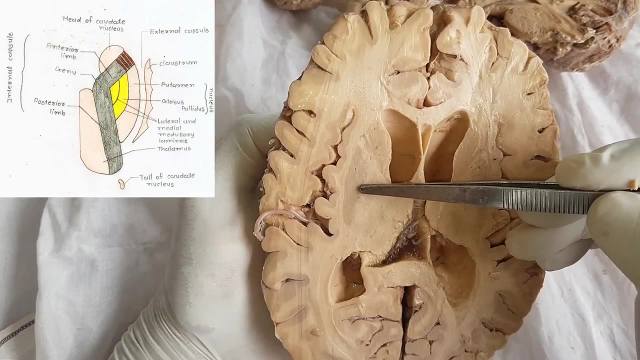 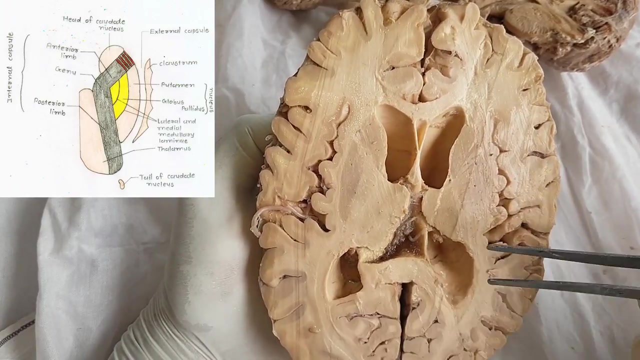 by this external medullary lamina, which is thin sheet of white matter, into the outer segment, here known as the putamen, and inner segment is the globus pallidus. and this globus pallidus again divided by internal medullary lamina into the outer segment and inner segment. 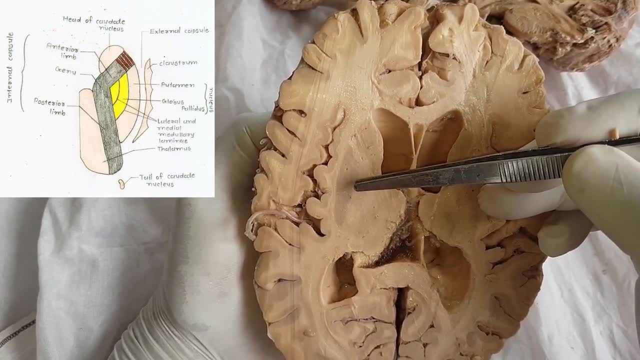 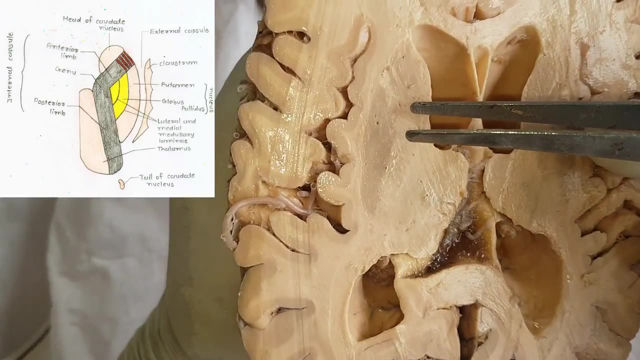 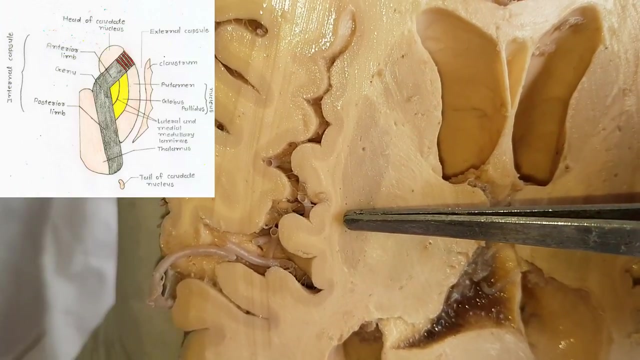 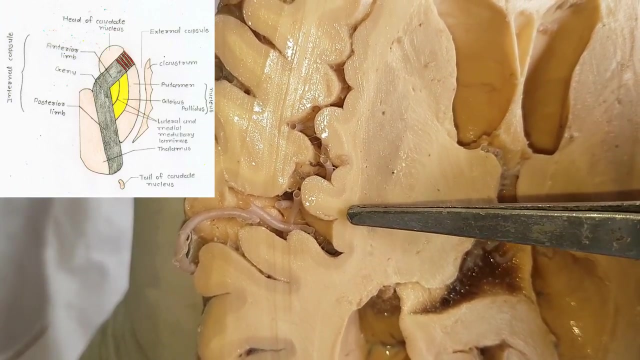 but in this section we cannot see clearly this globus pallidus and its outer and inner segments. Now this lentiform nucleus. on close inspection you can see This is lentiform nucleus and another thin sheet of gray matter. you can see thin sheet of gray. 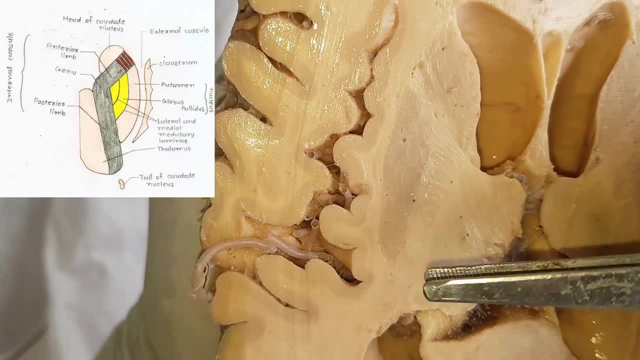 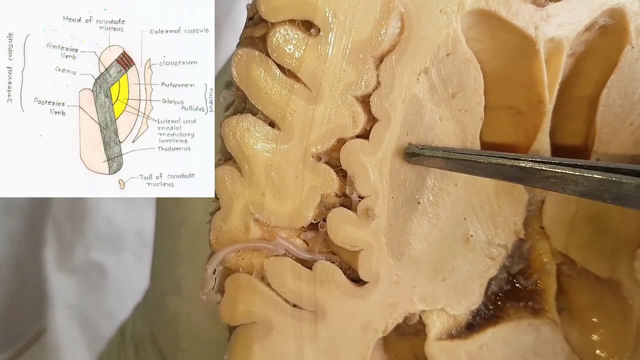 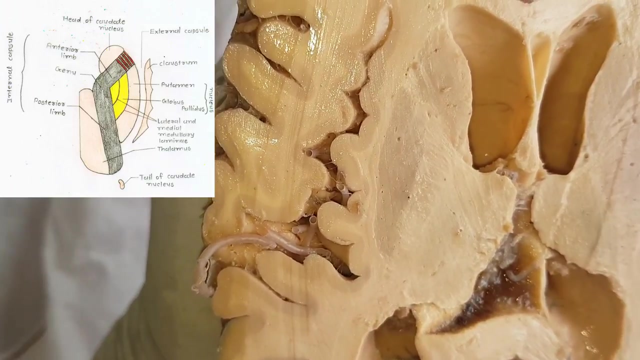 matter outer to this lentiform nucleus is the claustrum, is the claustrum so, and this claustrum is separated from this lentiform nucleus by the thin sheet of white matter known as the external capsule, and this claustrum, thin sheet of gray matter. 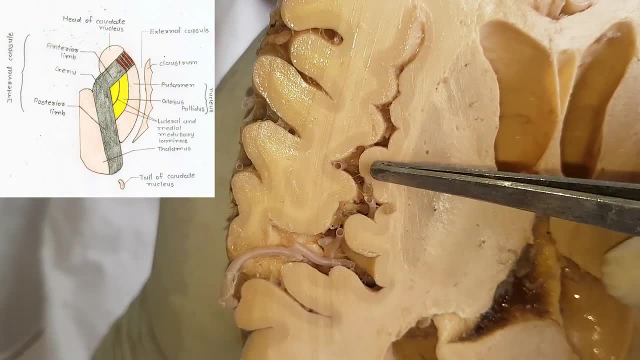 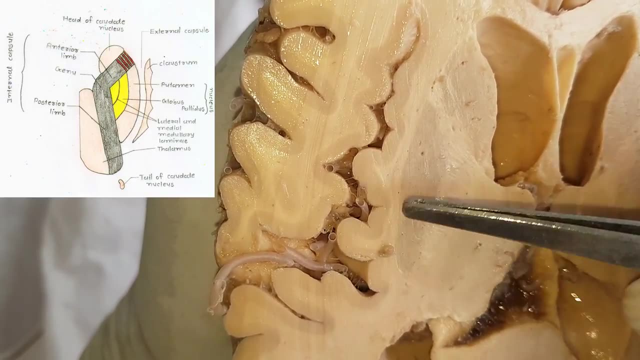 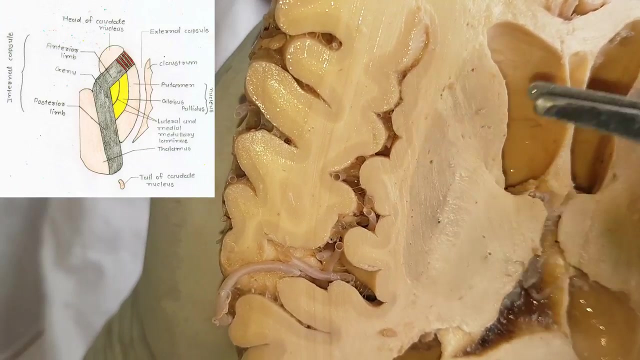 is related literally with this insula. this is the insula, an insular cortex. but this insular cortex is separated from this claustrum by another thin sheet of white matter outer side. this one is known as the extremy capsule. extremy capsule- clear. here are thewaribe. 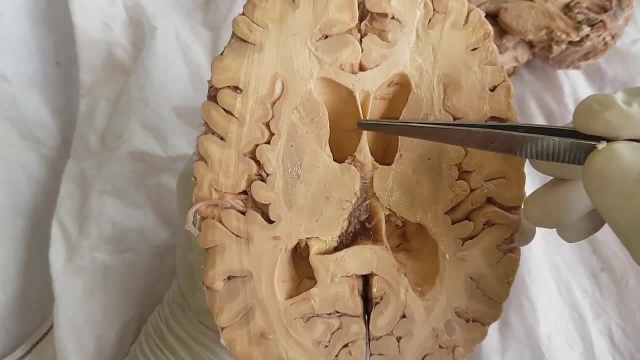 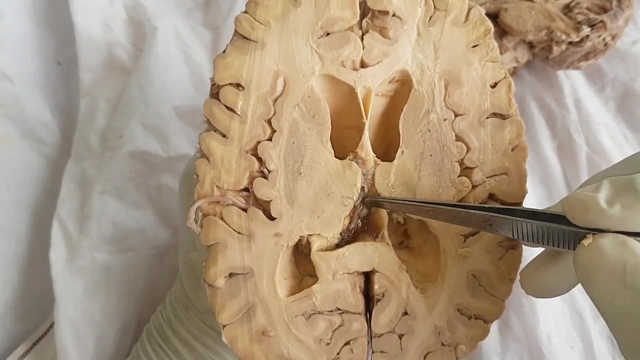 metals and we can see the cloacstrums and cluster of administer by another thin sheet, major forceps, minor cavity of lateral ventricle. both side, this is the septum pallucidum. this is the cavity of third ventricle. on each side are the thalamus: this is the caudate nucleus. 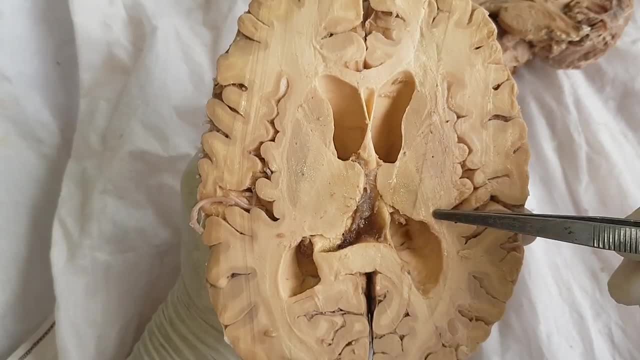 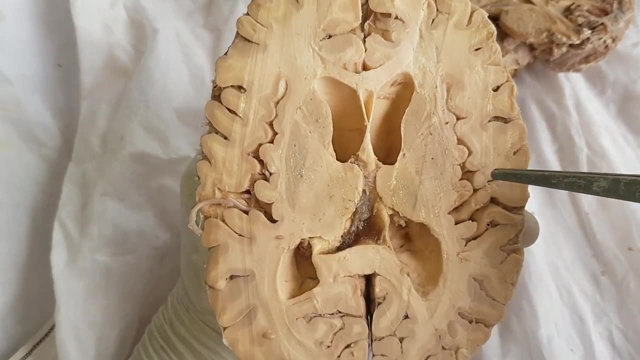 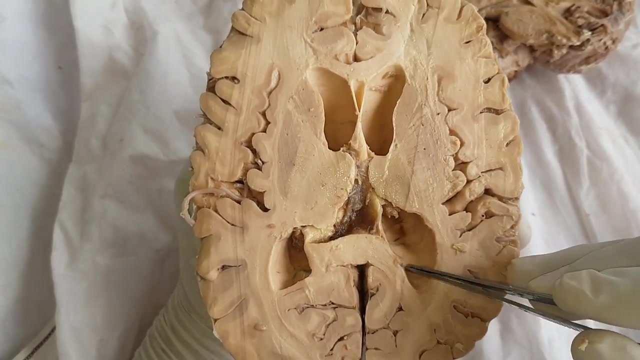 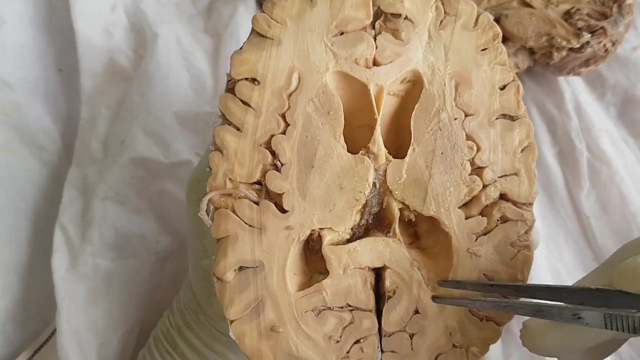 and v-shaped on both side is the internal capsule. this is the lentiform nucleus and claustrum and the insular cortex on both side. here you can see the posterior horn, just lateral to it. you can see this white fibers on both side. you can see clearly this white 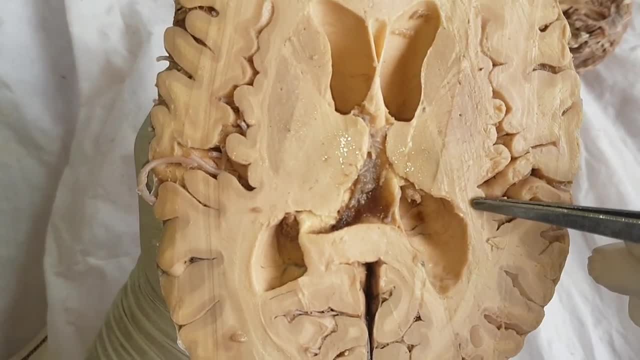 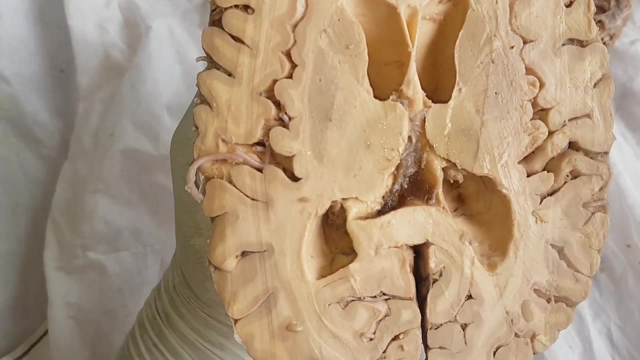 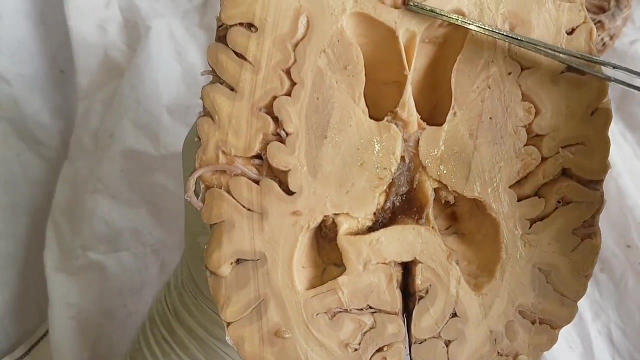 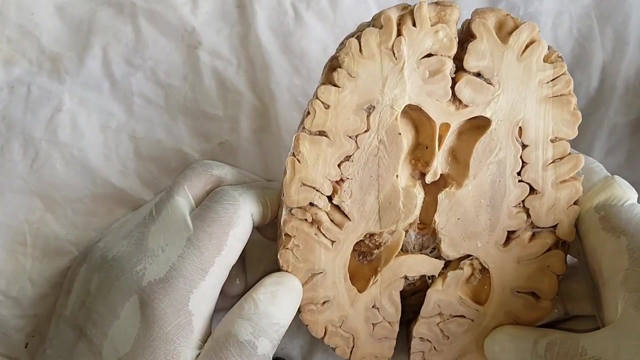 fibers are the fibers of optic radiation which extend from the lateral geniculate body. so this is the transverse section at the level of genu and the splenium of corpus callosum. so this is all about the various sections of the brain. thank you, if you like our video. 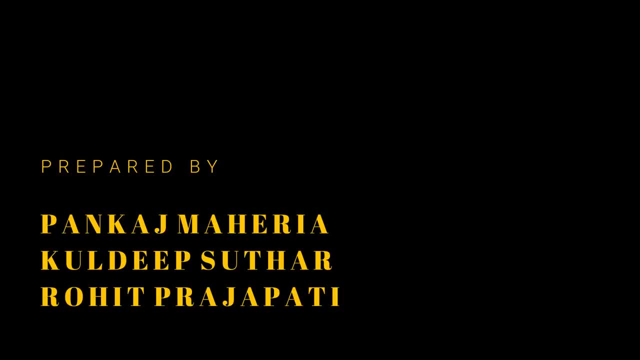 click on the like button and share with your friends to get the regular updates on anatomy video by viva boss of anatomy. subscribe to our channel and click on the bell icon to get the regular updates on anatomy. Hello everybody, I wanted to spend a little bit of time talking about how to find the intersection points of two polynomials. We're going to do it graphically, which is a really short thing, And then, more importantly, I want to show you how to do it algebraically. 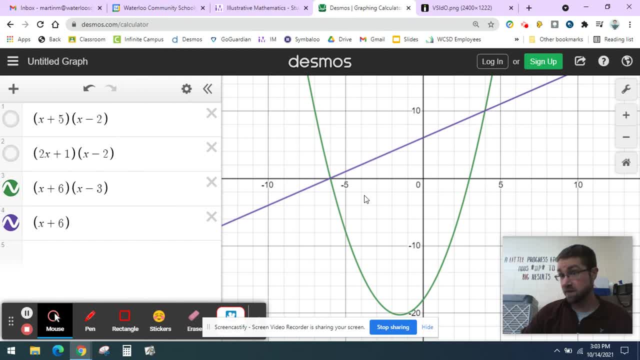 because I know that's a little trickier. Okay, So if you want to find the intersection points graphically, you graph both of the polynomials and then you look and you try to find the places where they're crossing. So there are two intersection points for these polynomials. 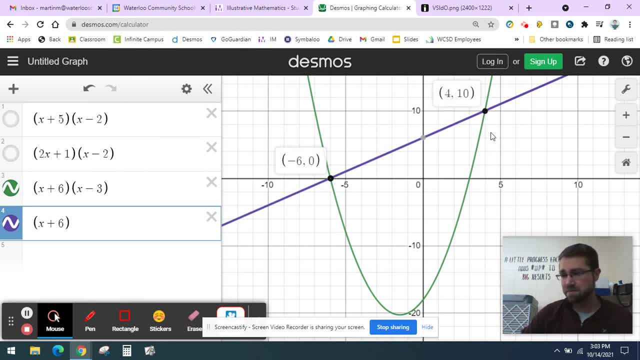 at negative, six, zero and four comma 10.. Now you might ask: why do the polynomials cross over at those specific points? And the reason would be: if I plug in the x value, that is, if I put in four into either function, I will get the same output, which is 10.. Believe me, You don't have to believe.